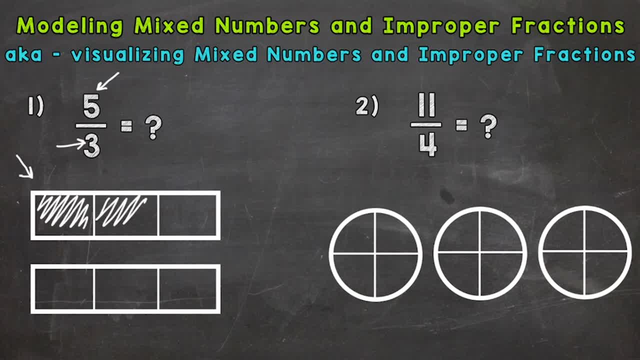 one third, two thirds, three thirds. So three thirds is three out of three. So that gives us one whole rectangle: four thirds and five thirds. So that model matches our improper fraction of five thirds. Now let's put it into a mixed number. Now we do not need to do a separate. 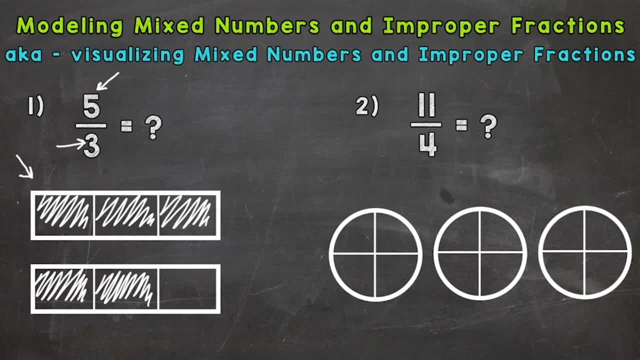 model for the mixed number. The mixed number is equivalent to that improper fraction. So we see that we have one whole rectangle filled in, So that's our whole number of the mixed number. Then we have one third, two thirds, So we don't quite have another. 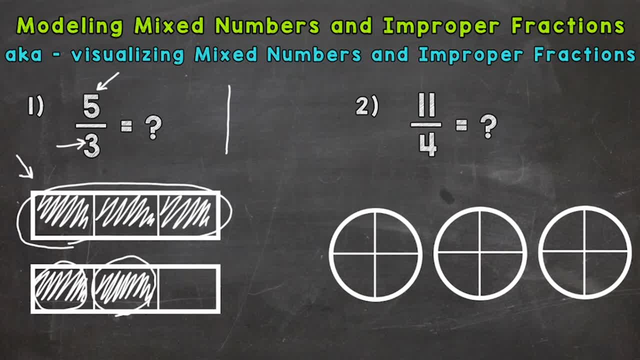 whole rectangle. but we have a fraction, So one and two thirds. And remember, a mixed number is a whole number and a fraction, So one and two thirds. Now, five thirds is equivalent to one and three thirds. They hold the same value. One's an improper fraction and one's a mixed number. Now you 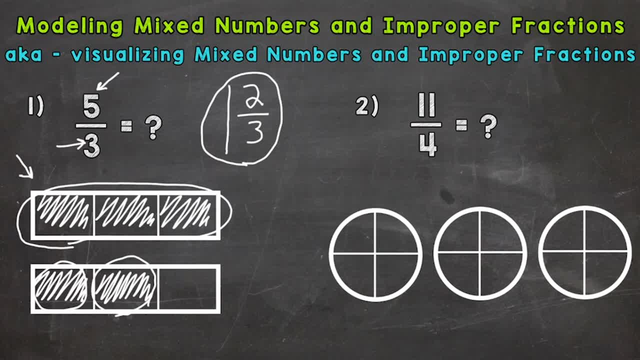 do not need to draw a model out in order to go from an improper fraction to a mixed number. I have another video that shows how to do that. I dropped that down in the description. This video again is about modeling mixed numbers and improper fractions. So let's move to number two, where we 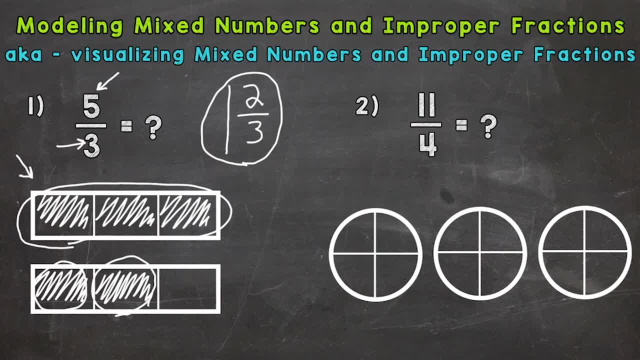 have eleven fourths. So I have some whole circles down below Cut into fourths So we need to fill in eleven fourths. So one fourth, two fourths, three fourths, four, fourths, So we have four out of four, which is equal to one whole Five fourths, six. 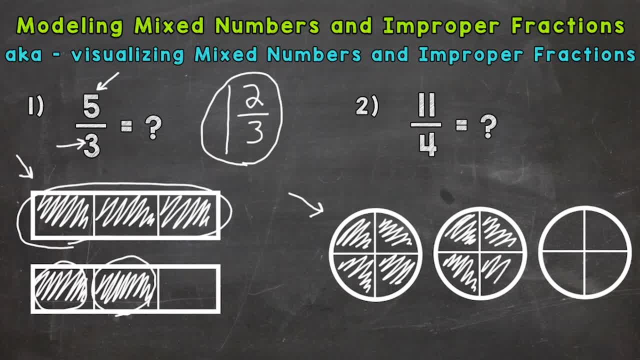 fourths, seven fourths, eight fourths, which is equivalent to two wholes- nine fourths, ten fourths, So that model represents eleven fourths. Now we need the mixed number, So we have two whole circles filled in. So that's going to be our whole number for our mixed number, And then we have one.